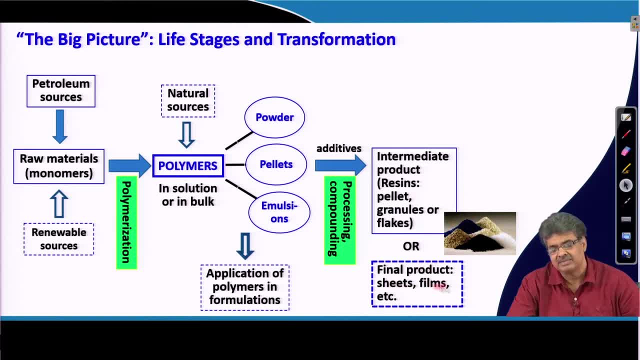 are very simple shape, like sheets, films, pipes, etcetera. Once we are ready with this intermediate product, then these are taken for production. Now further processing. in this step we can add additives and do a processing which is called designing, fabrication, finishing to get the final product. 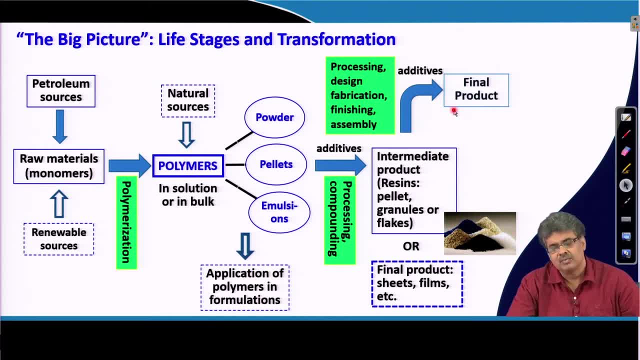 Now, in laboratory we do not actually make final product, these are done in commercial lines. So to basically estimate the product performance in laboratory, some specific samples are produced having a well defined geometry and testing are done with those samples to and this testing data are correlated to the final product performance. 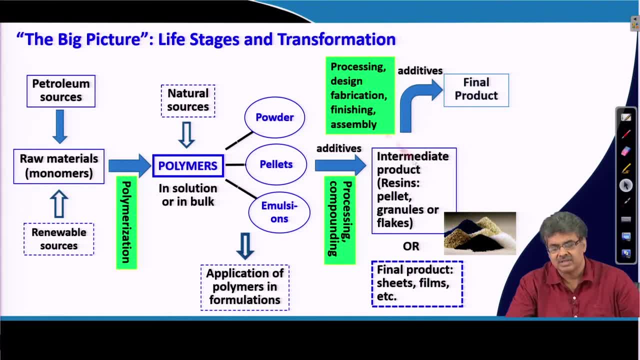 So the entire steps or these steps, which basically takes the polymers which are synthesized to the final product formation. these steps are collectively called polymer processing. Now I want to also make a point in this slide that generally polymer producers or polymers manufacturers, they do not actually shell the final product. 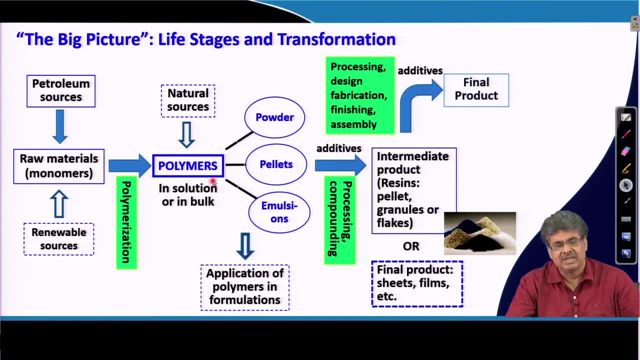 For example, company like Bayer which makes polycarbonate. they do not sell the final product of a DVD or CD or a car headlamp or so on. So company like Bayer's what they do? they synthesize polycarbonate and sometimes they 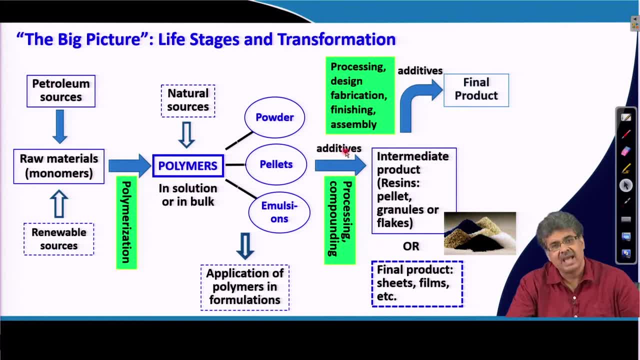 sell the powder, or sometimes they add different types of additives to make different grades of polycarbonate and then sell in the market. and there are other companies which buy from Bayer and further process it to make the final product which goes into the final application. ok, 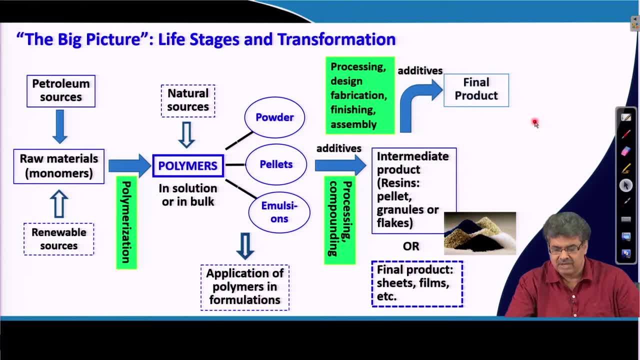 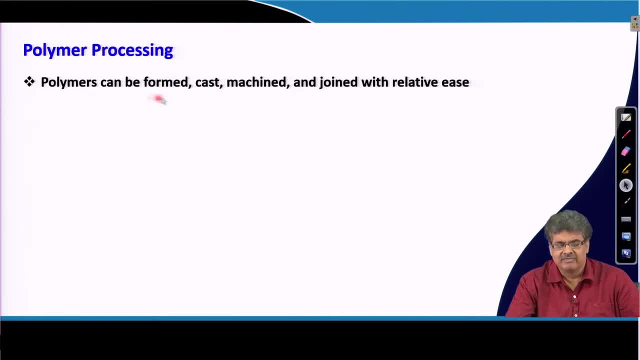 So now I will move the polymer processing brief. polymers can be formed, cast machines and jointed with relatively ease, and it requires little or very low amount of post processing or surface finish operation. Polymers melt or cure at relatively lower temperature Compared to, say, metal or a ceramic and as a result, polymers require lower energy to. 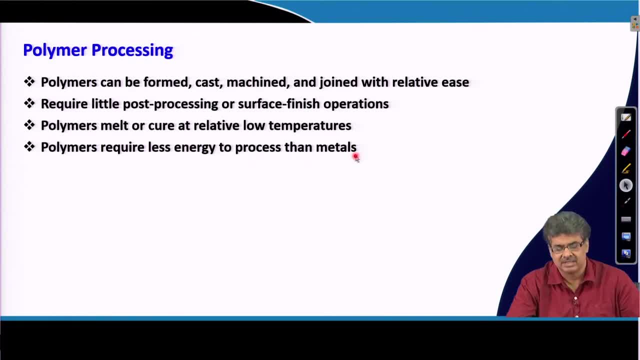 process compared to those materials like metal And polymers are used to make reinforced composites. Basically, the other reinforced mains are done by adding some other components in the polymer mixture. These are not very easy to do with materials like metals and ceramic, And generally polymer process starts with the raw materials, which are commonly polymer. 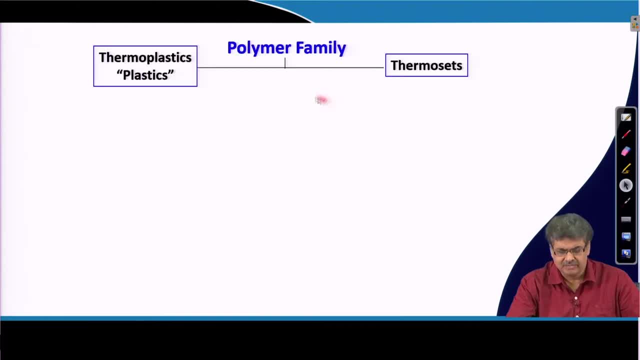 pallets or polymer powder. Before you go into the polymer processing steps, we just revisit the polymer families, because the type of processing Which need to be followed or the condition which need to be followed during processes depends on the type of polymers that need to be processed. 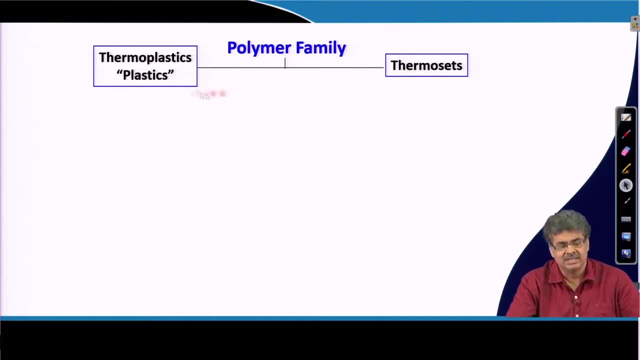 And generally we have two types of polymers, as we discussed earlier: thermoplastics, which can be reformed after melting, and thermosets, which we cannot reform. Thermoplastics can be either semi crystalline or amorphous, And thermosets can be elastomer or glassy. 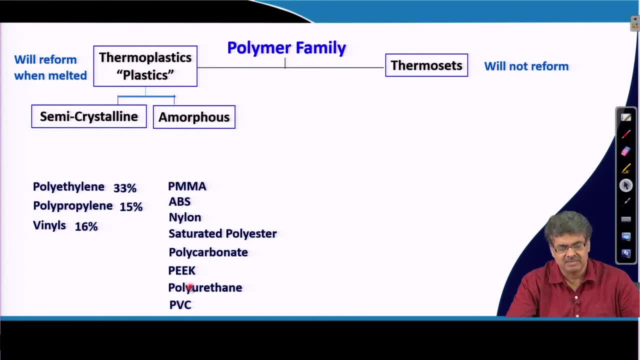 These are some of the examples of semi crystalline and amorphous polymers, And these are some of the examples of thermosets polymers. looking at the polymer, we need to basically determine the condition of polymer processing or the type of polymer processing we need to. 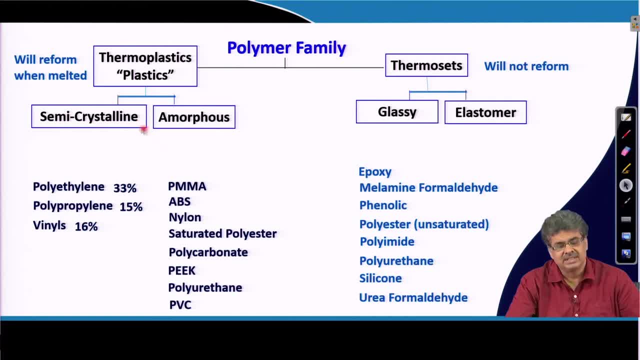 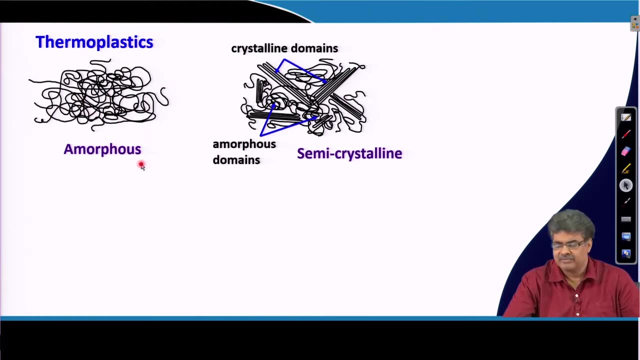 So thermosets polymers can carry with the knowledge that what type of polymer This particular which somebody has chosen to process is. Thermoplastics are two types, as we said: amorphous or a semi crystalline polymer, which contain both crystalline and amorphous region. 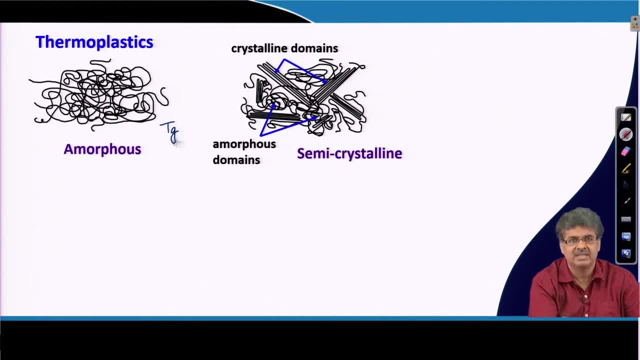 Amorphous polymers are characterized by polymer. What is a crystalline crystalline, polyester, polyester polymers. There are two types of polymers of amorphous characterized by a temperature called glass transition temperature, and semi crystalline materials are characterized by 2 temperature melting point, which are related to this crystalline. 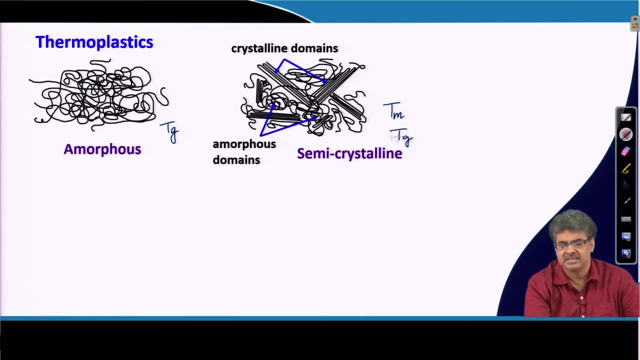 domain and Tg, glass transition temperatures which are related to this amorphous domains. So we need to have a understanding of the values of these Tm and Tg to set the processing temperature. These are crosslinked material thermoplastics and 90 percent of the polymer markets are thermoplastic or consist of thermoplastics. 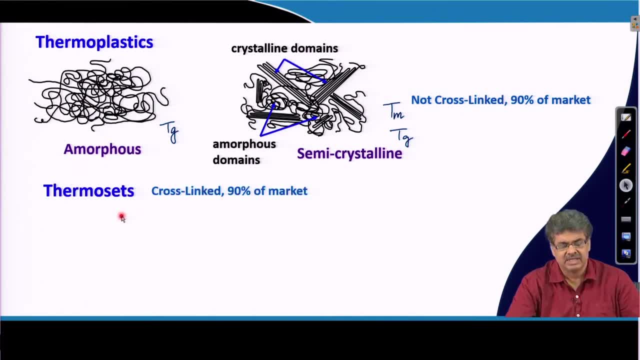 material, The other materials, as I said, The other material is thermosets, which are crosslinked and this mistake- 10 percent of the market is- this is 10 percent of the market- is made up of thermosets, And thermosets could. 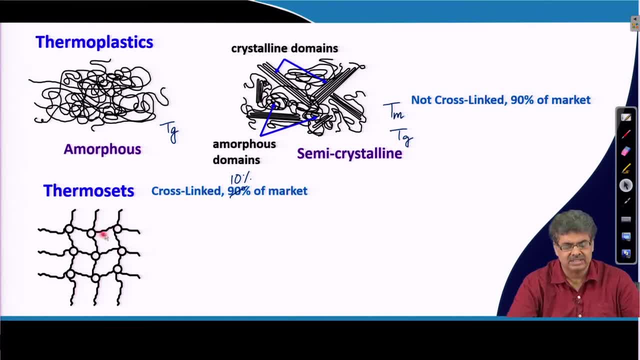 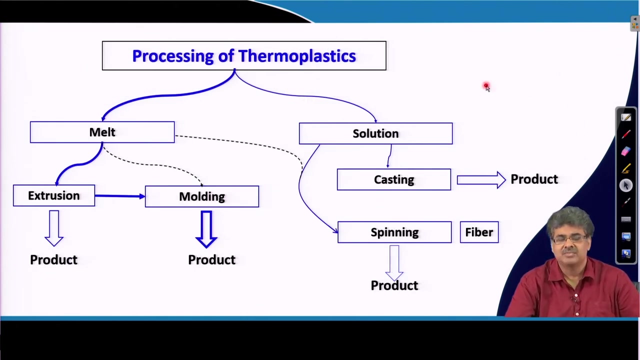 be 2 types. if the polymer chains, if the temperature of applications is below the glass transition temperature or Tg of the. So some of the products are from from the extrusion step itself, but most of the products are prepared or manufactured after in the molding step. A part of or a minor part of 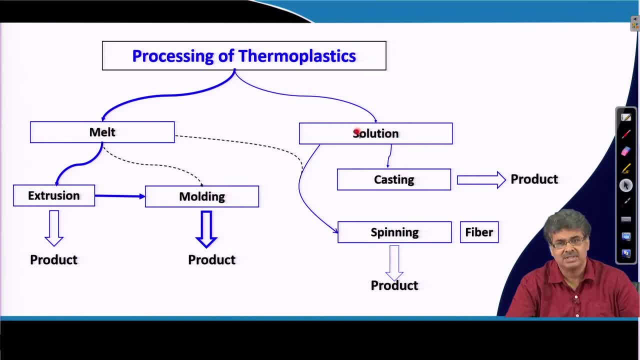 the processing is done in solution. that means the process polymers are dissolved in solution and then cast it to make products like film, Or it is spun to make products like fiber. Sometimes this pinning can be done with the molten polymer as well, but the extent or the weightage of that process is much lower. 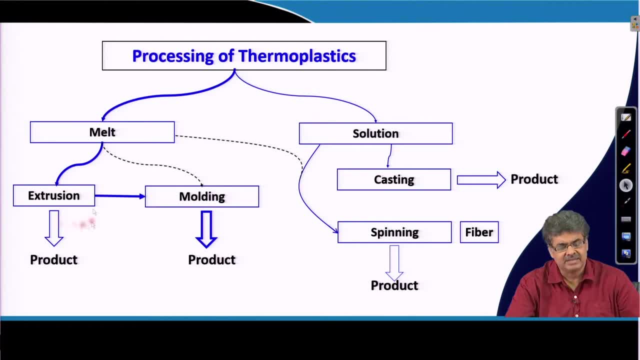 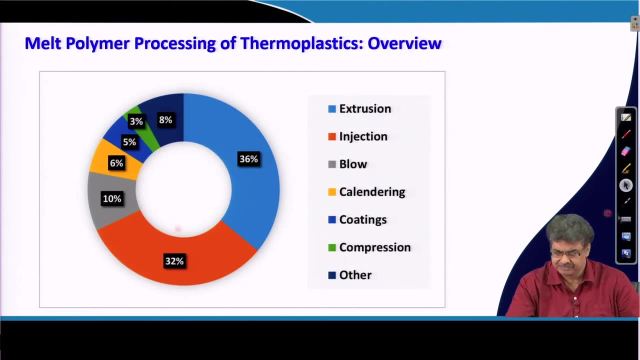 So we will mainly discuss the extrusion process and various types of molding process, because those are the most important or most abundant Polymer processing steps done for synthesizing polymers product. This is the basically what is the extent different products are formed like. most of the products are formed either. 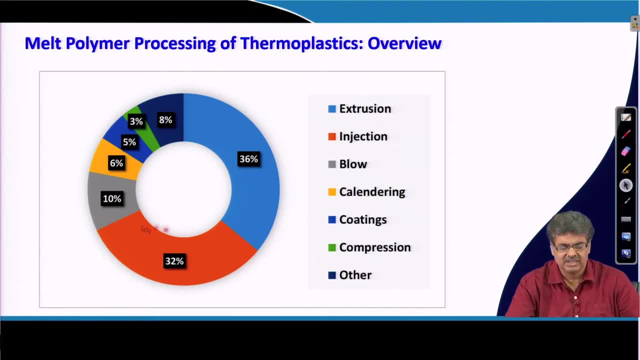 by extrusion or by injection molding. Some products are formed using a process called blow molding and there are other molding process process which responsible for the other other type of product formation. So we will talk mostly about few of these important processes like extrusion, injection. 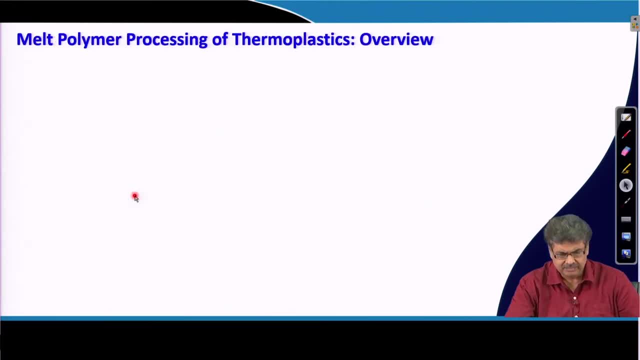 molding, blow molding and so on. So in processing of thermoplastics, first step is we basically mix the polymer and then add different types of additives. we can regrind or we can make a master batch of additives and add this here and we basically mix it in this step and then we take it to next step. 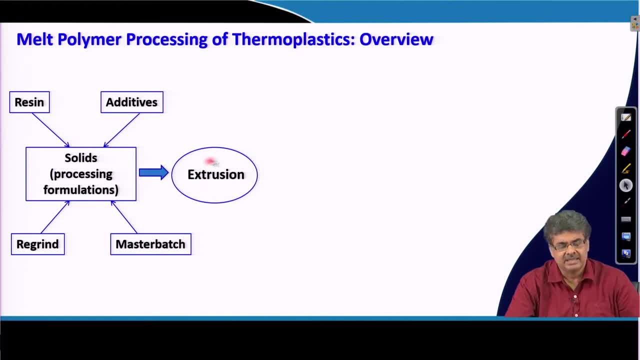 basically melt it And do a step called extrusion and, as I said that, from this extrusion step itself we can make some products like pipe and sheets. but in most cases this extruded products are followed by a second step, molding step, to make most of the products. and in this step, in this molding, 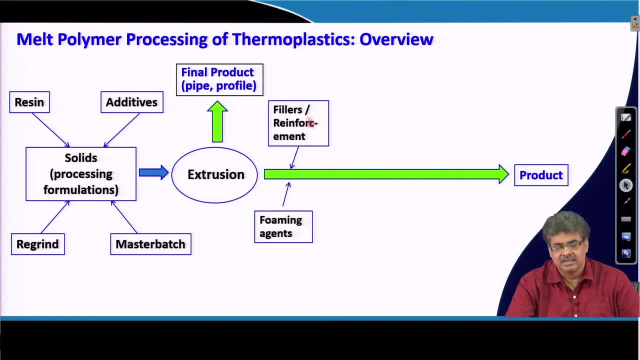 step, we add other. So now, so after preguntas are assuming exactly what I have shown here, you start to ask more questions. ah, If you do construct like proper third order and then the third order, then you do like a secondary three code. forgive me to keep you silent. remember, I have shown the Glossary. 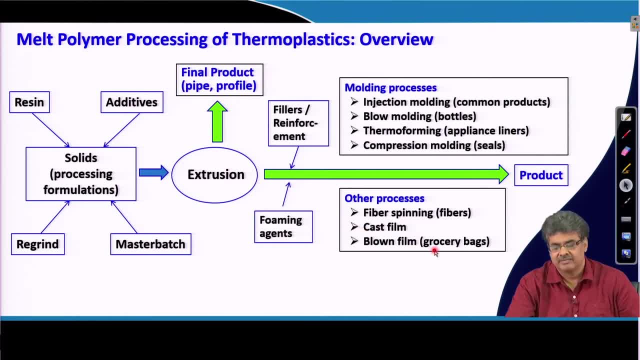 bag process for drying of theinetilene. So the the method with complete cleaning principles. This will not serve the ind academia, so this is a는데요 thing, So we will associate all to 얘기 you about process development. 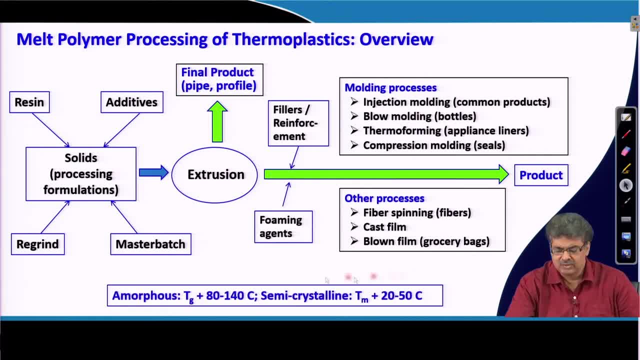 Bah, Then we will precisely have azoomrisk to all the components, like fillers, reinforcement. This is a general rule- is followed that for amorphous material the processing temperature is typically between Tg plus 80 to Tg plus 140 degree. 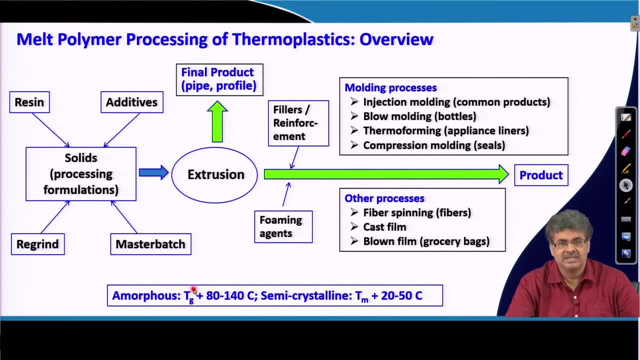 So if the polystyrene is having a glass transition temperature of 100 degree centigrade, then polystyrene is generally processed between 180 to 240 degree centigrade. A polycarbonate which has a glass transition temperature of 150 degree centigrade it is. 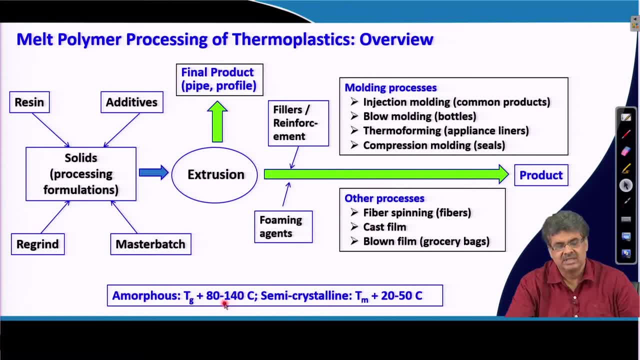 generally processed at, say, 250 or 270 degree centigrade. Similarly, for a semi crystalline material, the processing done is above the melting point, 20 to 50 degree centigrade above the melting point If the temperature is taken too high. 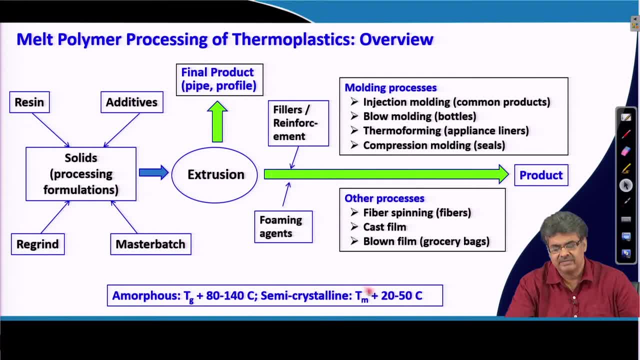 Then obviously viscosity will be too low. it will be difficult to process. Similarly, if the temperature is too low, then the viscosity will be very high. then it will be also difficult to process. So this is a typical window of temperature in which, or at which, the polymer processing. 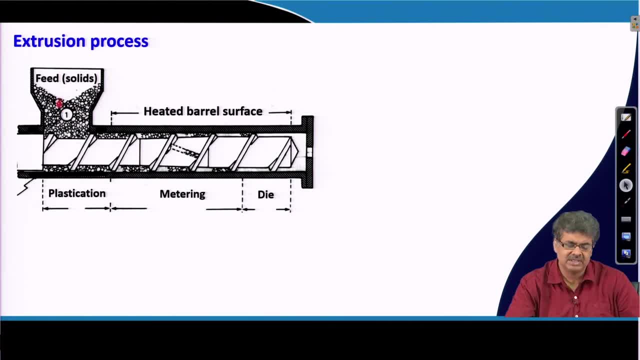 is done So in the extrusion process. this is a cartoon of a extrusion machine. So screw inside sometimes a single screw, or it could be a two screw. we call twin screw extruder and this is a orifice which we call as a die. 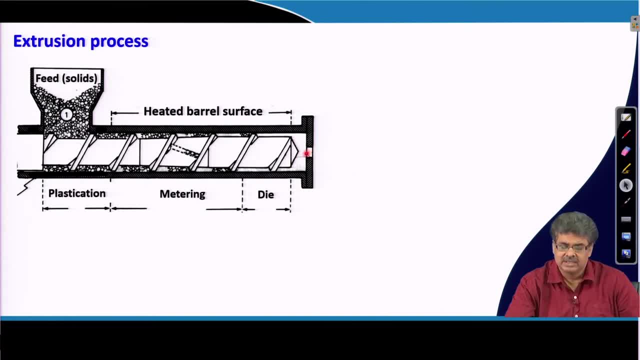 So from here the product is basically taken out and the shape of the die will determine what shape of the material or processed extruded polymers which are coming out. You can have a Sheet type shapes, where you can, or a pipe type, like circular die, where you can directly. 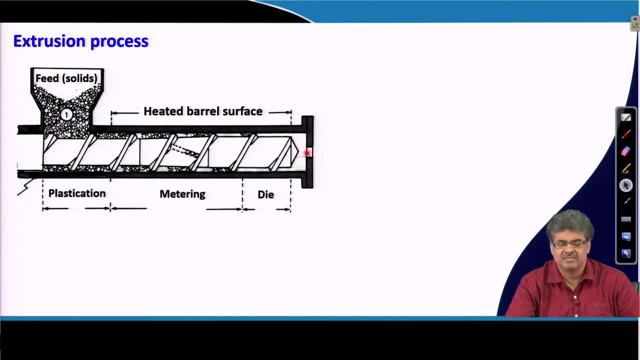 get extruded pipes or sheets or otherwise, you can have a small orifice by which you can get a long polymer strands and you can chop it, cool it and chop it to get small granules. So in this case there are 3, 4 regions. 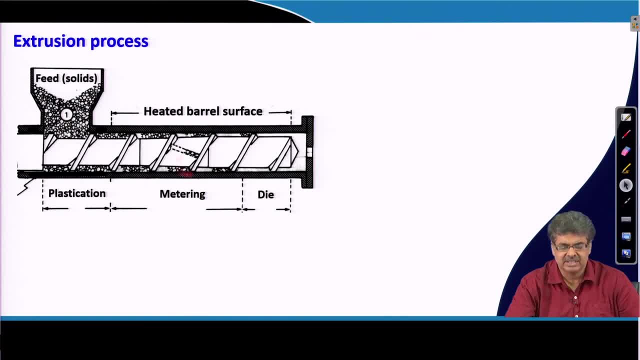 This is a feed region, this is the plasticization region and this is a metering region and this is die region. So I am not going in details. what is the role of each region, because that is out of scope of this course. but in this case the temperature is slowly increased from left. 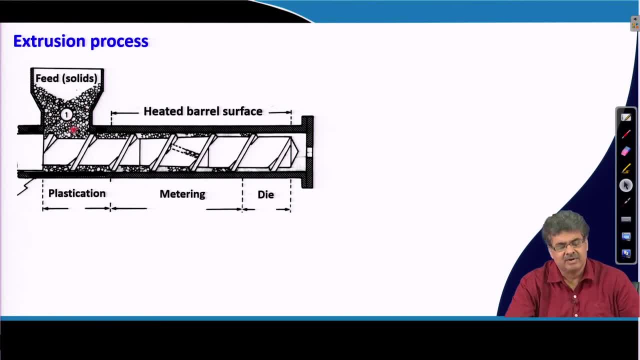 hand side to right hand side and the polymer science. polymer samples are melted here and pushed by this screw And through this dies. this is the most common manufacturing for plastic. resin, as I discussed earlier, combines pigment additive and resin. it is a high heat process and high pressure. 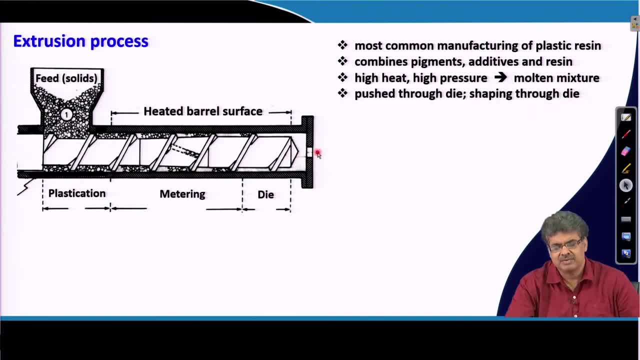 process molded mixture. in this process, the extruded products are pushed through the die- and you can use different shapes of the die as well- and it creates warm plastics For further finishing operations like palletizing, calendering or molding, as we discussed earlier. 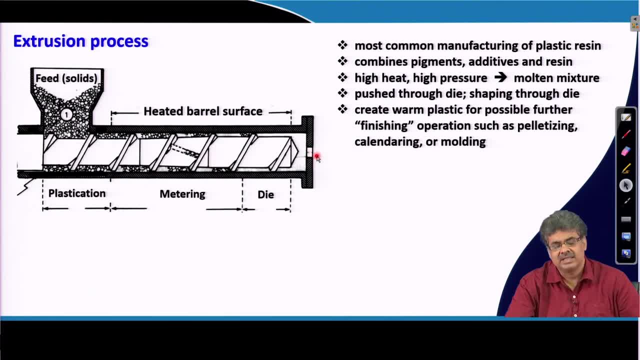 so it basically gives the materials for further processing- the second step which we discussed earlier. So it basically pumps the high viscosity melt. it also mix different ingredients. You can actually use this also as a reactor. If we use this as a reactor, we can also use this as a reactor. 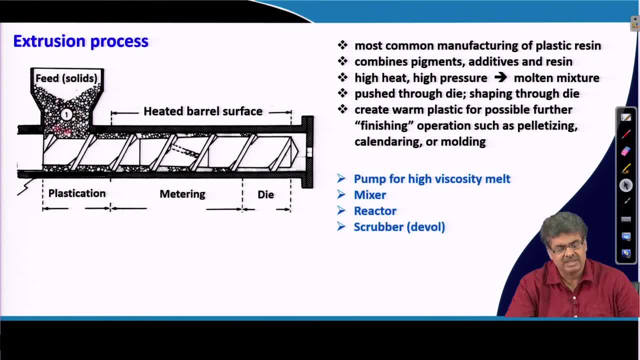 So this is the process. We can also use the materials which reacts with each other, which is not very frequently done, but we can do that. We can use this extruder as a reactor also, and it can be used as a scrubber as well. 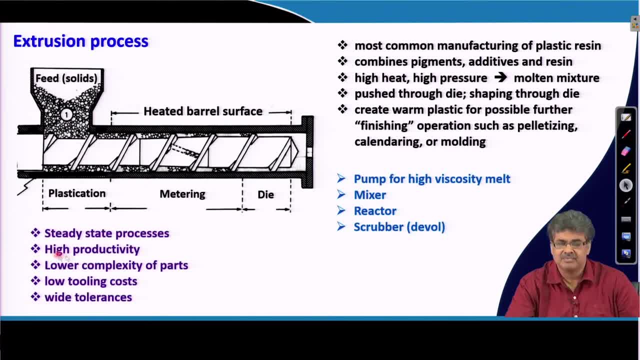 So it is a steady state process: high productivity, lower complexity of the parts which we can generate, low tooling cost and wide tolerances. So this, that is the reason it is very powerful. So this is the process. So this is the process. 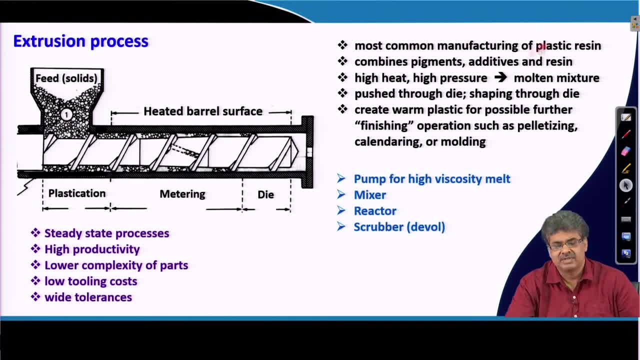 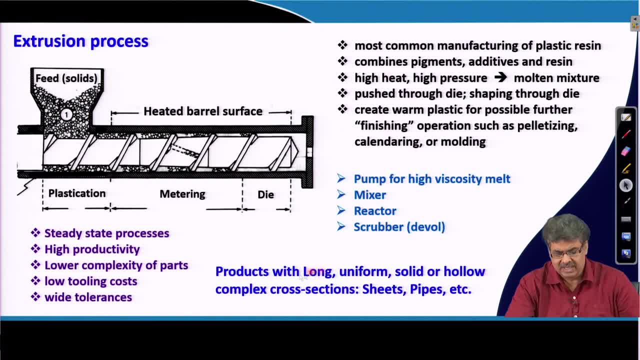 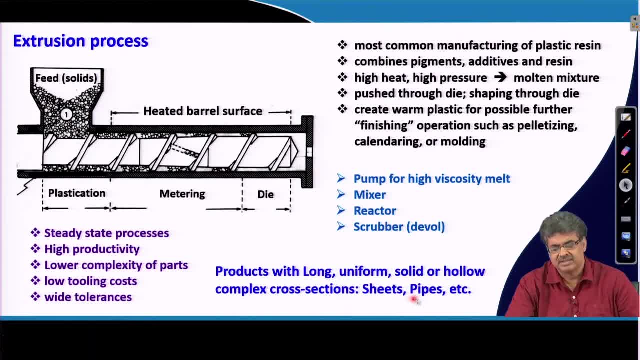 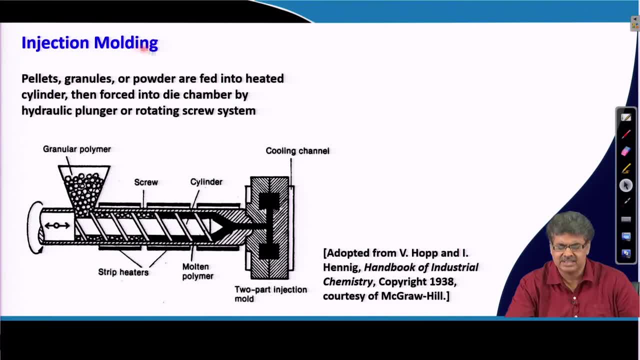 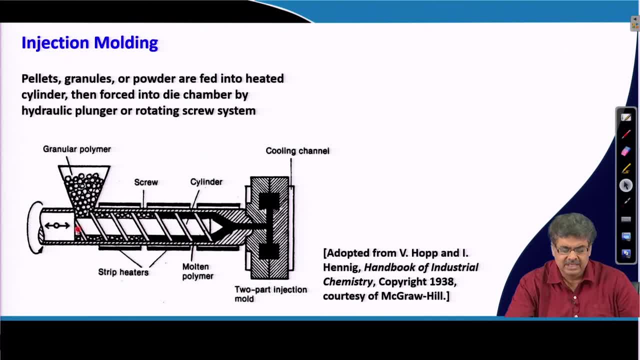 a injection mechanism. this melt is injected to a cavity which is having a particular shape, depending up on the final product shape, what we require, And this is done with the help of a screw and, once the in the, this molten polymer is injected into the cavity. 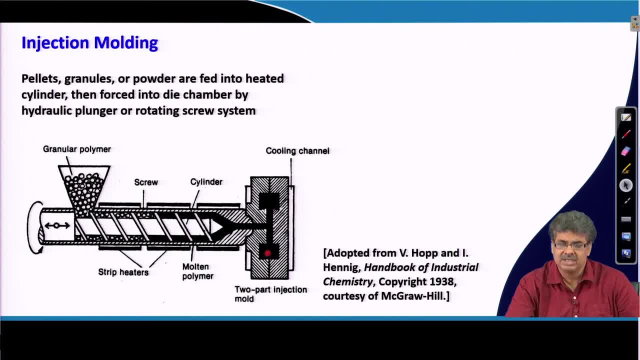 it is cooled So that it is the shape is frozen and then it is taken out from this cavity and we get the product. In this case, a dog bone shape sample is produced here which are typical used for mechanical testing, which we will discuss later. 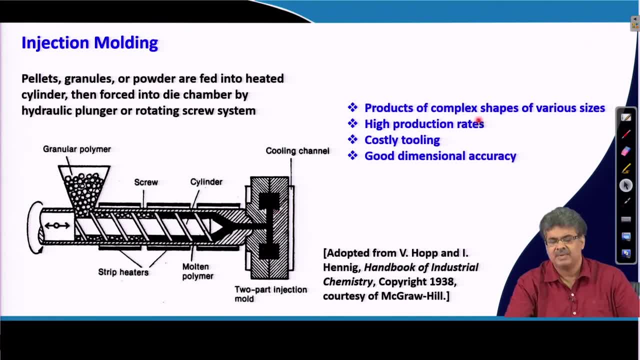 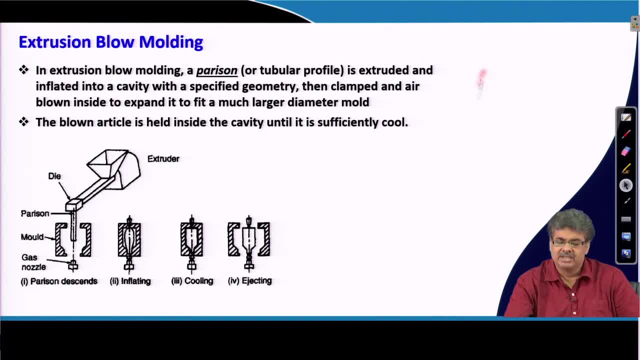 In this case, the like, the hollow products are generally PPS, like this water bottle, water storage bottle. and in this case, what is done? a partition which is a tubular profile which is extruded using a extruder and then it is placed in a cavity where it is inflated using 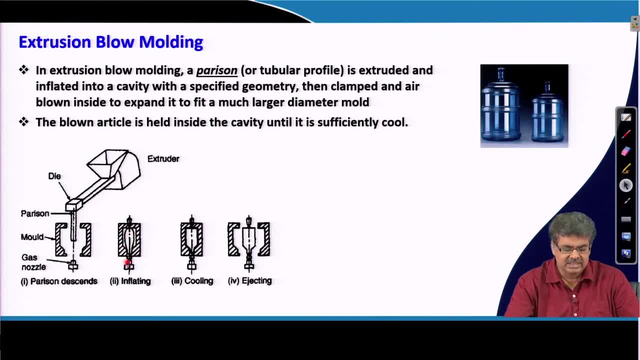 a inert gas and once the inflation is complete, like it basically covers the entire shape of the mold which we are using here, like a bottle shape here, and it is cooled and then, once the cooling is done, complete, the shape is frozen, then we can take out by removing. 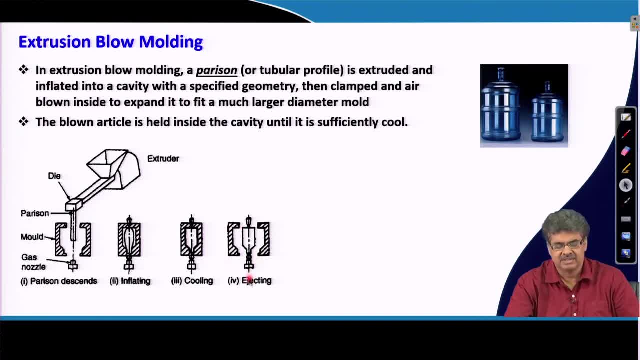 this molds And cutting it from here, which is called ejection process. So in this case this type of products are produced, So this can be a continuous process. hollow thin wall parts of various sizes can be synthesized, produced in this extrusion blow molding processes high. 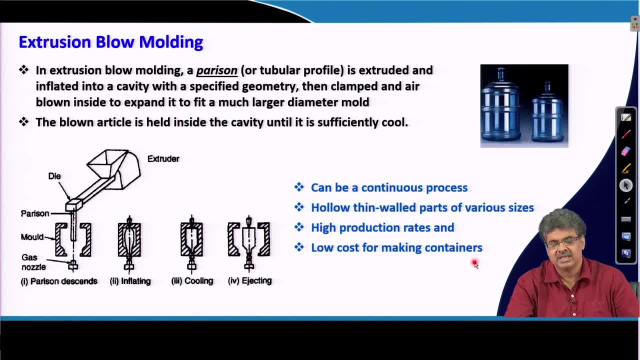 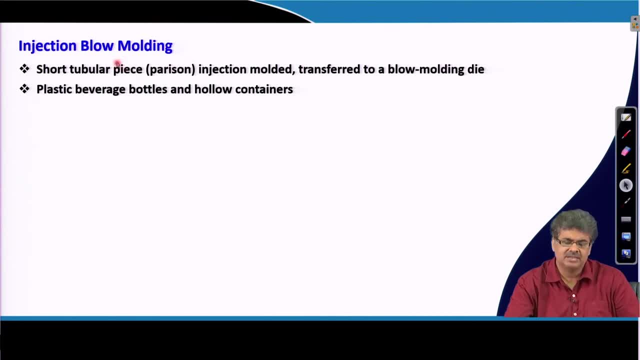 productivity rate and low cost for making containers. We can also have others type of molding process which I will quickly go through, like injection blow molding in case short tubular piece or partition, as we discussed earlier for extrusion blow molding, their injection molded and transferred to a blow molding die and the rest of the 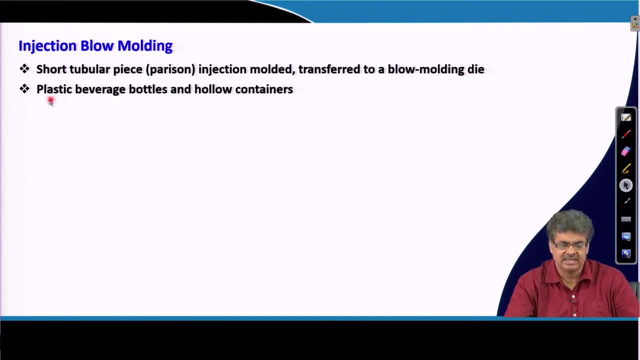 process followed exactly what I discussed in last slide. Plastic beverage bottles or hollow containers are generally produced using this mechanism of process or this processing step: Multilinear blow molding. we talked, we discussed blow molding and, in this case, the polymer which are used like the extrusion, in the extrusion we extrude. 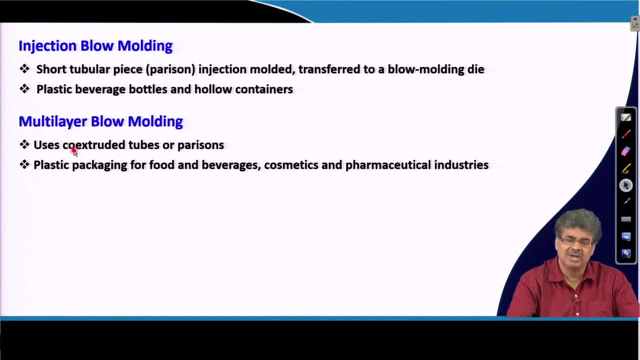 co 2 layers. So basically extrude two or more layer, one after one, and then, using the same process, we can make multilayer plastic product which are used for packaging material. Multilayers are necessary to use for different purpose, like barrier and hydrophobicity oil repealing. 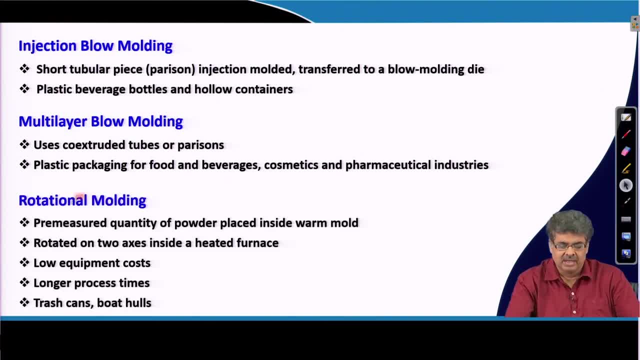 and so on. Rotational molding, in this case pre measured quantity of powder sample is placed inside one mold and then rotated on two axis inside a heated furnace, and it has low equipment, cost longer process time and products like trash can bowl boat hulls can be used by this type of molding. 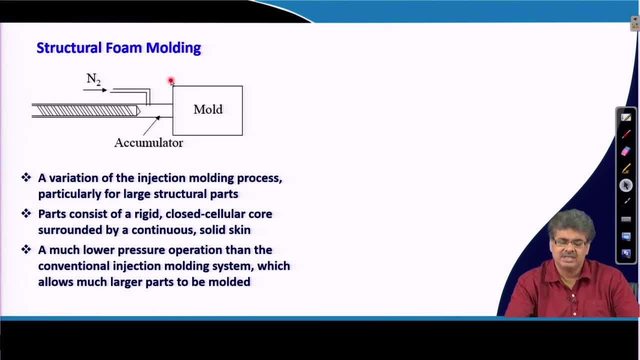 So structural foam material, which are just little modification of the injection molding process, in this case during the injection process. gas- inert gas- is also used for the injection molding, basically added or injected along with the polymer melt. So the polymer melt will now content this inert gases in the molded product it produced. So in this 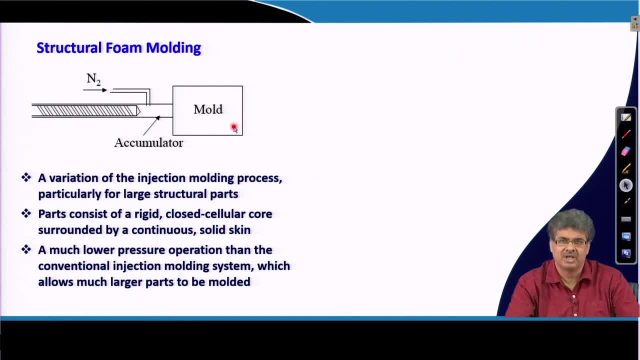 case. basically we call, now we discuss. we are making a foam product where gas are dispersed within the polymer matrixes. So it is a variation of injection molding process, particularly for large structural parts. Parts consists of a large and close cellular core. means that gas or this gas core, surrounded by continuous solid skin of polymer. 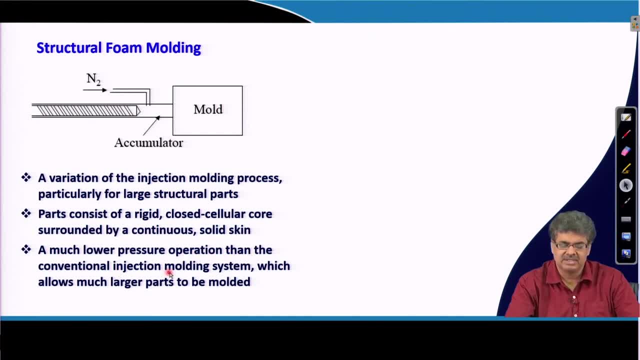 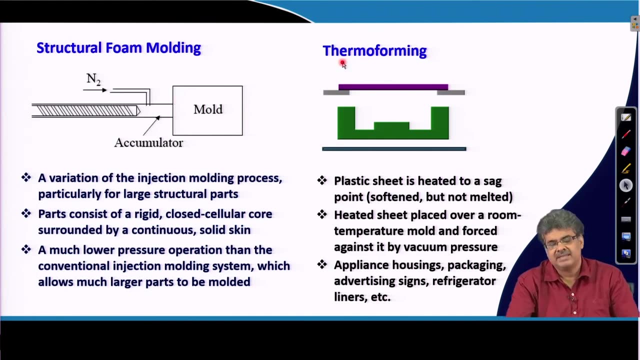 A much lower pressure operation than conventional injection molding system, which allows much larger part to be molded, in this case, conventional injection molding system. So this is the case compared to a conventional injection molding process. Next, we will talk about thermoforming. as the name suggest, we basically in this case we 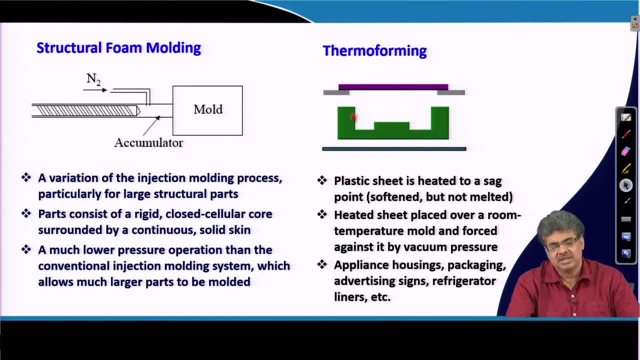 have a shape which is the shape of the product which we are planning to produce. These are used for products like tray and different packaging materials. So in this case, a film- polymer film- is heated so that it becomes soft, So it just heated. 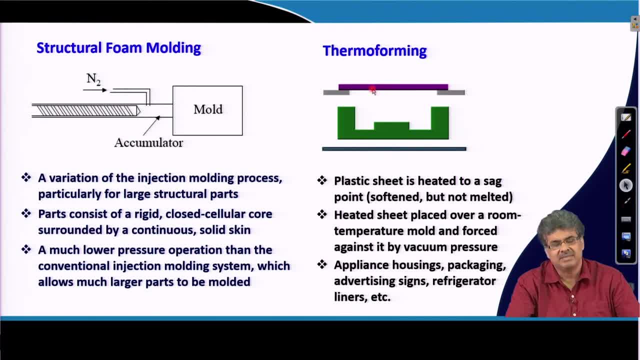 above the Tg or just above the Tm of the polymer- mostly Tg- and then vacuum is applied, so that now this film will basically form a shape of this mold, this mold, And once it is cooled this film will form a product like a tray, as in this. 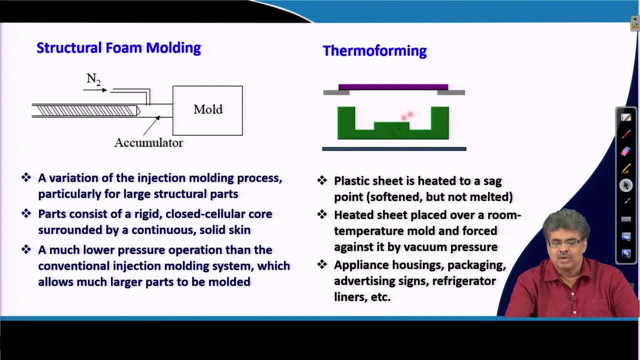 case it is shown here. So the plastic sheets is a sheet is heated to a sag point, like soften, but not melted, And this heated sheets placed over a room temperature mold. this is room temperature mold and forced against vacuum pressure. So basically vacuum is applied. 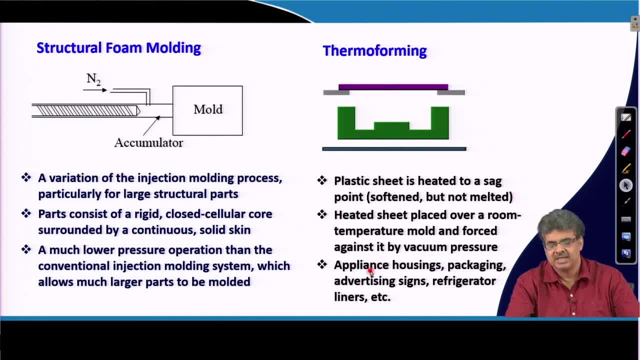 So it is forced on to this room temperature mold, and once it is cooled, then it will form a product of this particular shape. So appliances, housing, packaging, advertising signing, refrigerator liners, these are the materials which are produced using this thermoforming. 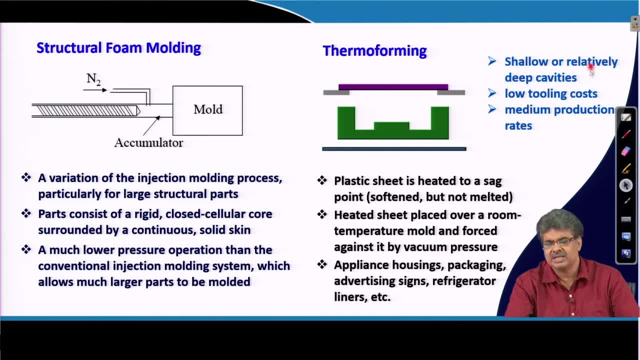 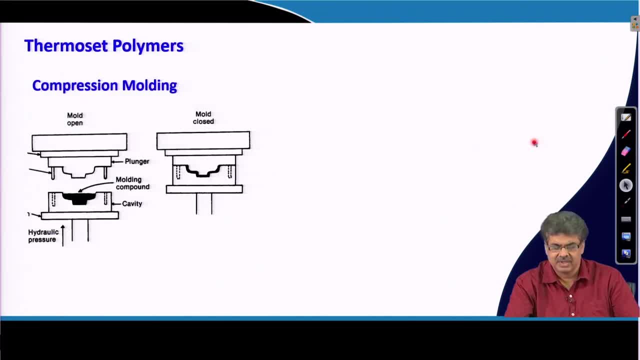 process. It is shallow or relatively deep, cavities can be formed. So these are the materials which are produced using this thermoforming process And it can be formed: low tooling, cost, medium protection rate. Next we will talk about the processing of thermosets, polymers, briefly, And most common process is compression molding. 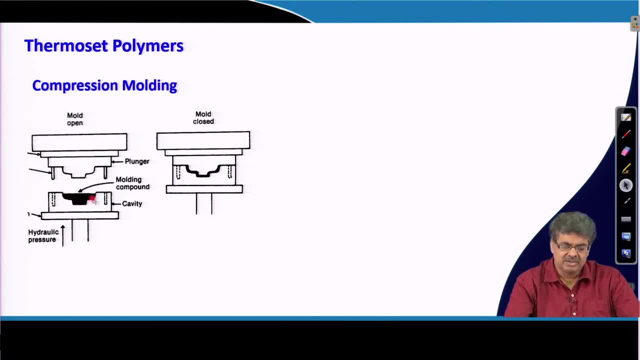 In this case the polymer, or a P polymer. just before curing it is placed into a cavity and agent it is heated to a molten, molten temperature and because it has a curing agent, So it might start cross linking and once it becomes soft, a mold is compressed on to this molten. 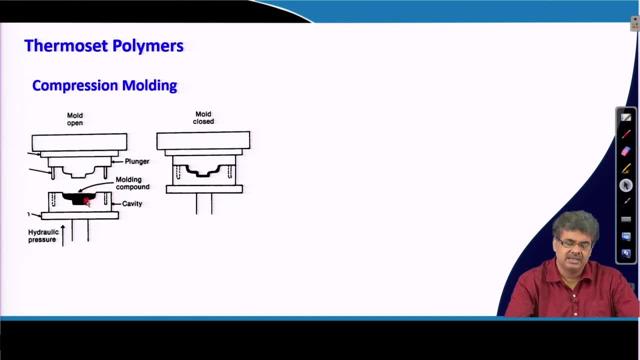 polymer and then it is allowed to cool. hence this product will form the shape of the mold as is shown here, and once it is cool, then it you can take it out by ejecting process. Another process we can do is reaction injection molding. this is used for chemical reaction. 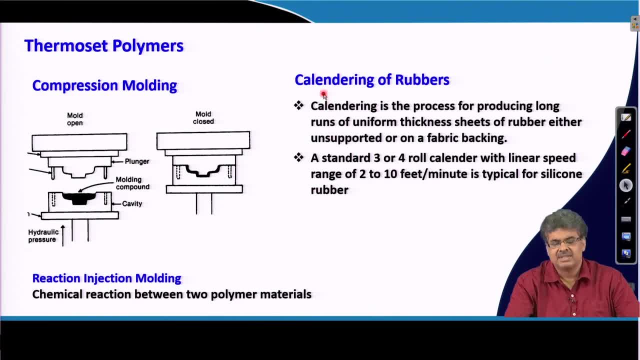 between two polymer metals. Rubbers are generally processed by calendaring processing step, called calendaring. in this case this is the process that produce for producing long run of uniform thickness sheets of rubber, either unsupported or on a fabric backing. So a standard 3 or 4 roll calendar with linear speed range of 2 to 10 feet per minute. So 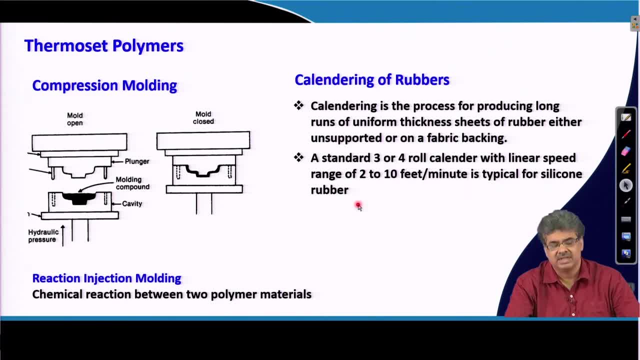 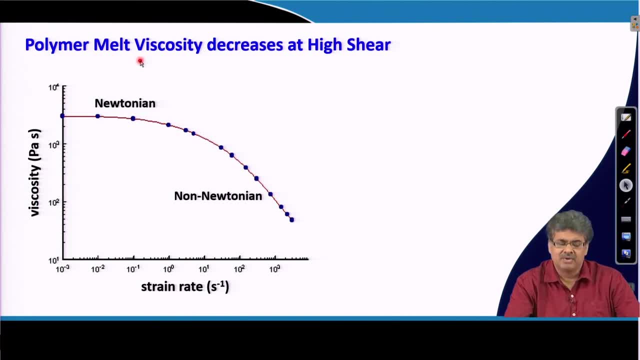 in it is typically for use for silicon rubber. Now, in case of polymer processing, as you now know that most cases the processing is done in molten state and polymers are very high viscous material. So in in molten state the viscosity will be very high. So injecting 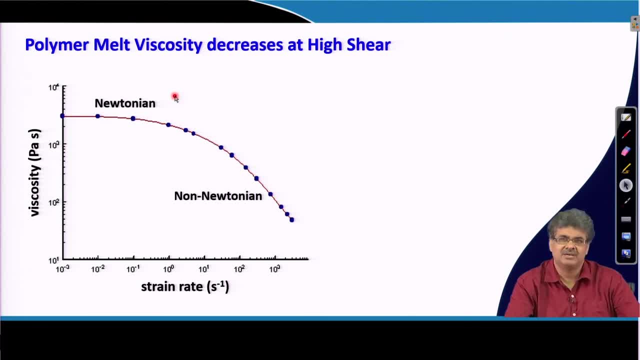 the material, or using material, Or basically pushing the material through a mold or through a die. it will be very difficult because of the high viscosity, but fortunately polymers are materials which are shear thinning, which means that at a high strain rate the viscosity of the polymer melt actually decreases. 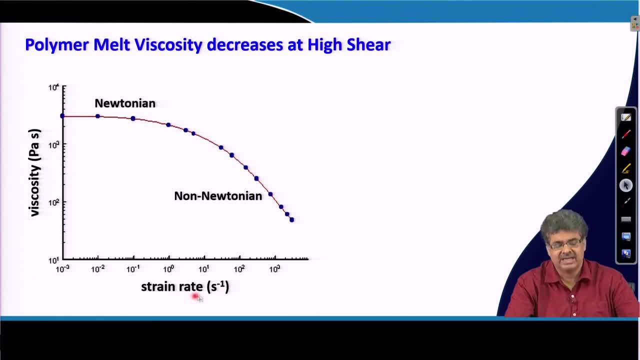 a lot. second inverse: Injection molding is the highest, having most high strain rate, like 1000 to 10,000. second inverse: So we now know how to make product different type of products from a polymer which has been synthesized by different processes. Now